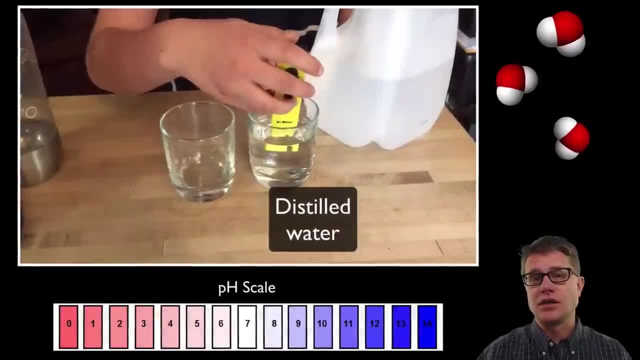 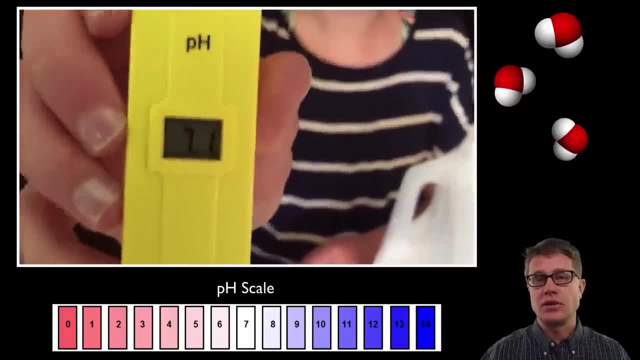 of carbon dioxide, But the mechanism is different. Let me show you a demonstration. This is regular distilled water And I am going to use a pH meter to measure the pH of regular H2O And it is going to be right around 7.. Now I am going to take that same distilled water. We 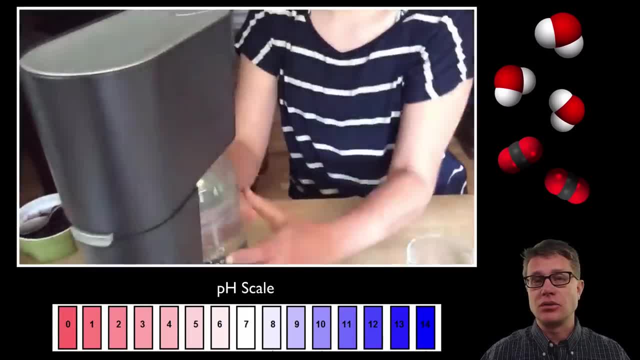 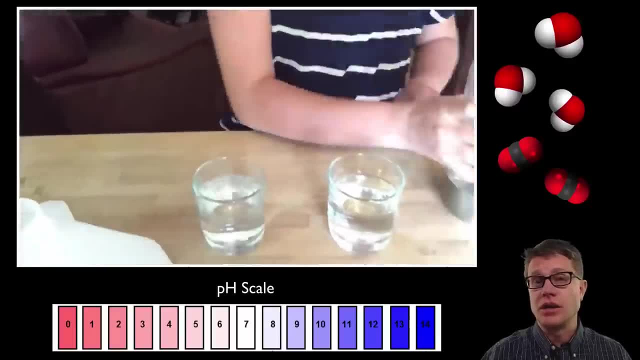 are going to put it in a bottle and we are going to add carbon dioxide to it. We are using a SodaStream machine to shoot carbon dioxide in it. It is now just carbonated water. We are going to put it in a glass and we are going to measure the pH. now I want you to 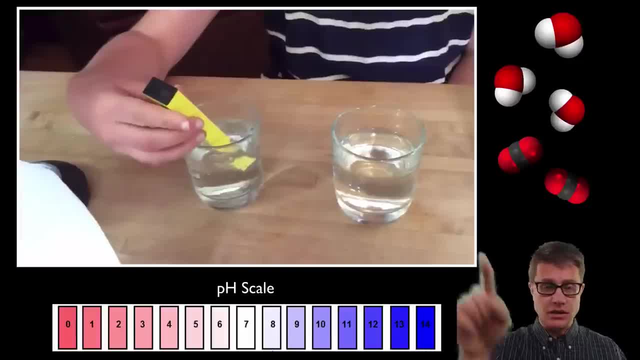 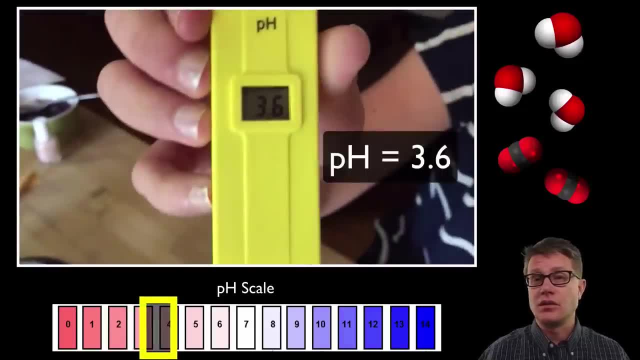 make a prediction of what you think the pH might be. You could even use your finger and point on the screen to where the pH scale is going to be. Let's see how you did. The pH is going to be 3.6.. It is really acidic. 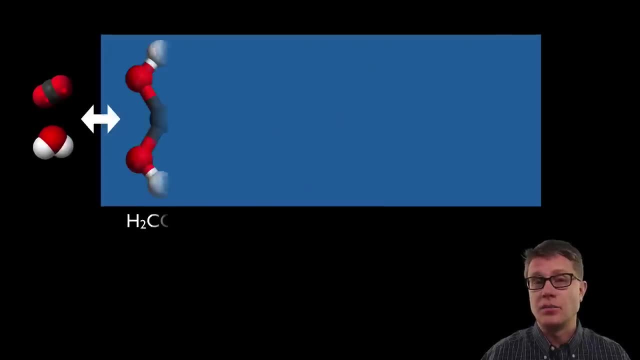 Let me show you what is going on. So if we take carbon dioxide and water and mix them together, we get carbonic acid. Now that can quickly dissociate and form bicarbonate. What we are doing here is we are losing one of these hydrogen ions And that can dissociate. 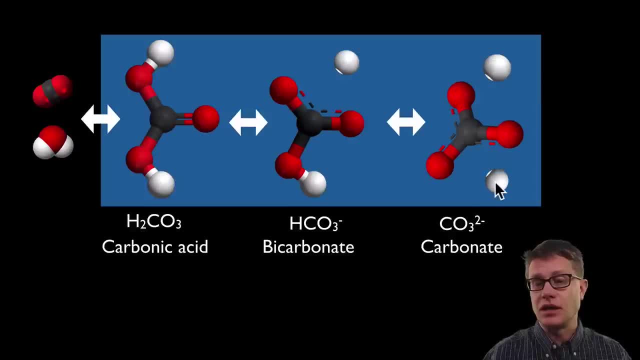 again and we can form carbonate. We are losing two of these hydrogen ions. Now, if we look at the definition for what pH is, pH, remember, is the negative log of the hydrogen ion concentration. What does that mean? The more of this H plus that we have in solution, the lower the pH. 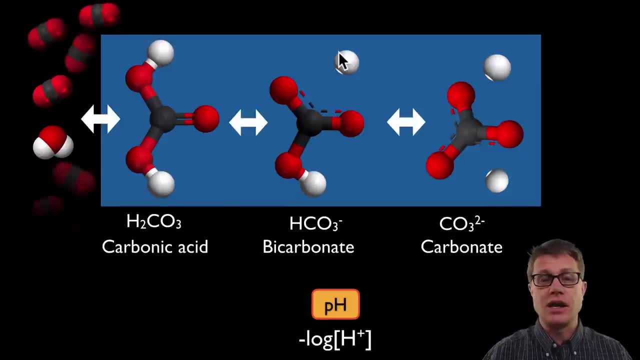 is going to be And the lower the pH is going to be. So if you look at the definition of pH, it is going to be more acidic If we add more carbon dioxide, more of it is going to move in and we are going to have more of this hydrogen ion and we are going to have 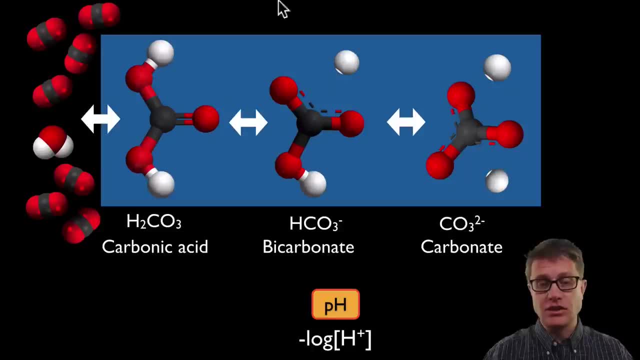 a lower pH. Now the levels of each of these can change. Each of these are reversible reactions, So, depending on the amount of carbon dioxide, it can move towards the left or it can move towards the right. Why is this a big deal? Well, life exists in this water And life is. 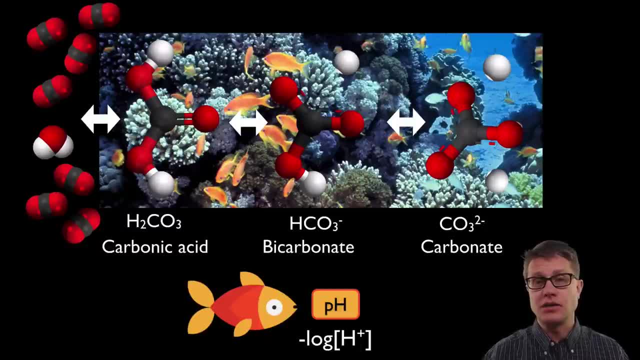 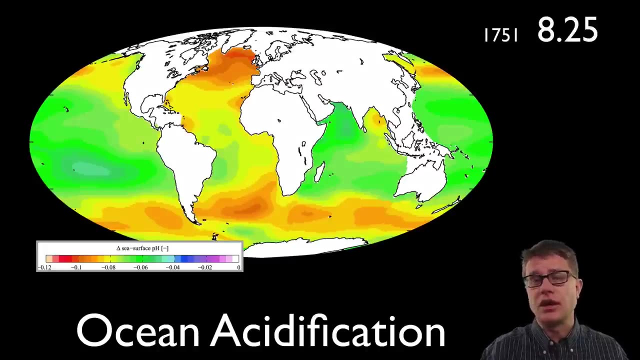 regulated by proteins, And proteins require a specific pH. So studies are showing that if we decrease the pH and make it more acidic, Organisms are having a decrease in metabolism and they can have a decrease in their immune response as well. Now how much of a change in pH are we seeing If we look at pre-industrial 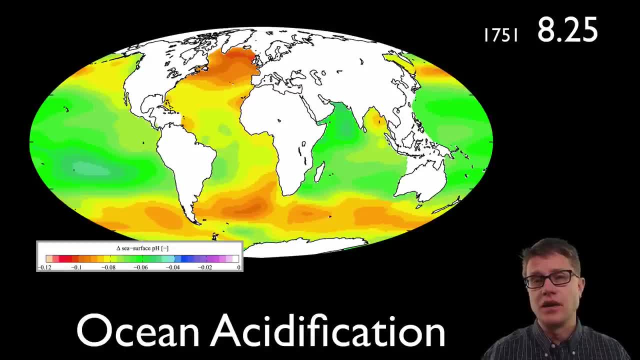 levels. the pH of the oceans was really basic: 8.25.. Post industrialization it had changed to 8.14.. Now there are going to be regional differences. you can see on this map right here And you might say that is not much of a change: in pH 0.11.. But remember this is. 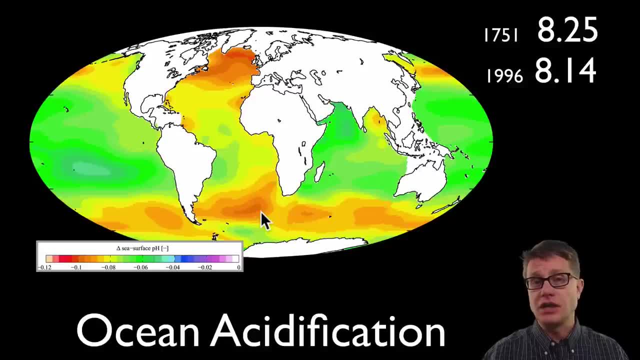 a log scale. So that represents a 30% change in the pH. What is it going to look like? What is it going to look like in the future? Well, as we play those models out into the future, by 2100 it could be as low as 7.80.. Now this low pH is going to devastate ecosystems. 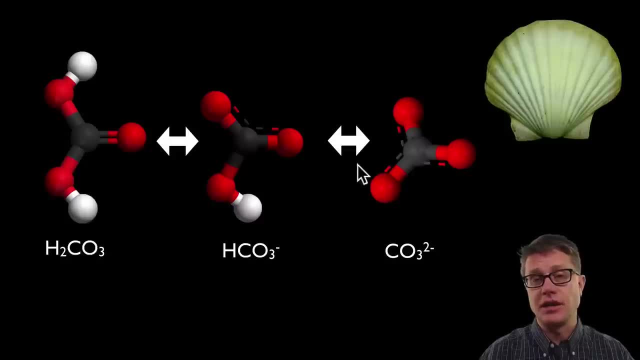 for a different reason. This last carbon compound of the three is carbonate That combines with calcium to form calcium carbonate. That is what the shell is made up of, That is what the bulk of a coral reef is made up of, And as we change the pH, we can change the level. 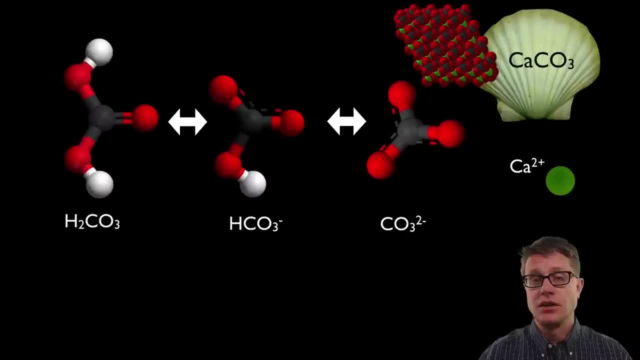 of that carbonate. What determines the concentration of these three? Well, it is going to be the temperature of the ocean water, the alkalinity- That is more than the pH that we need to get the wind water. the alkalinity, but also the pH, And so we can use a gerund plot to figure out. 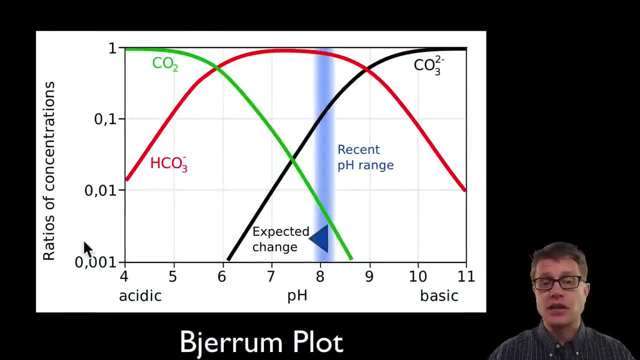 what is going to happen over time. These are log scales of the concentration of these three compounds. The green represents the amount of carbonic acid, The red line represents the amount of bicarbonate And then the black line represents the amount of carbonate. Remember. 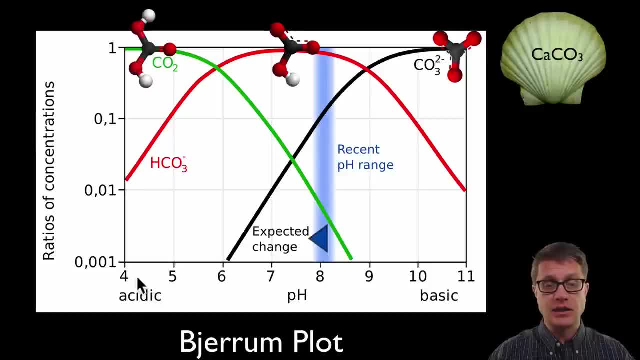 that is important for shells, And so, if we look at it at acidic levels, carbonic acid is going to dominate. At neutral levels, bicarbonate is going to dominate, And then at basic levels that we would find in the ocean, carbonate is going to dominate. But this blue area represents 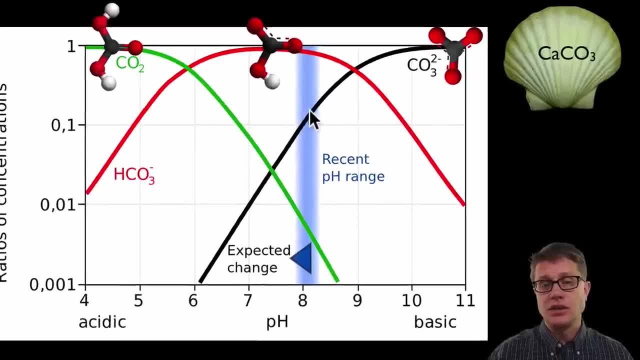 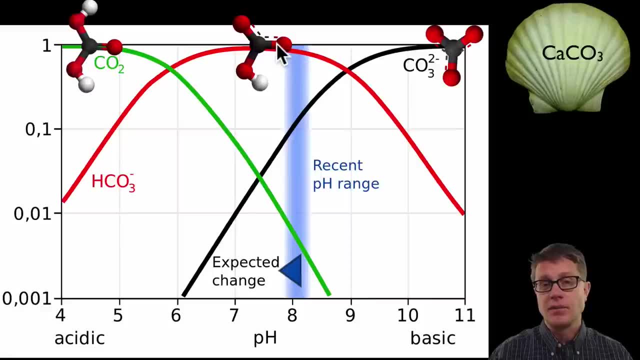 what is going to happen as we change the pH And as we decrease the pH. you can see what is going on: The carbonate levels are going to drop off and the bicarbonate levels are going to increase. That is because that free hydrogen is competing with the shellfish, really. 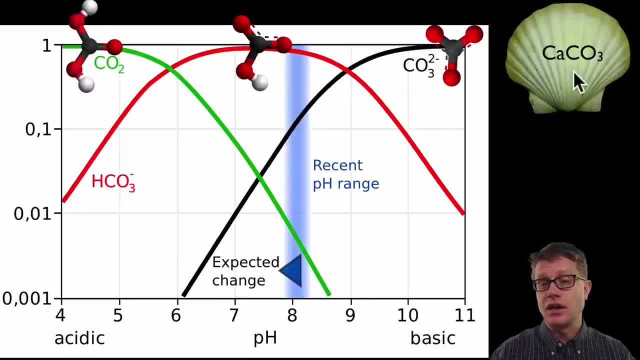 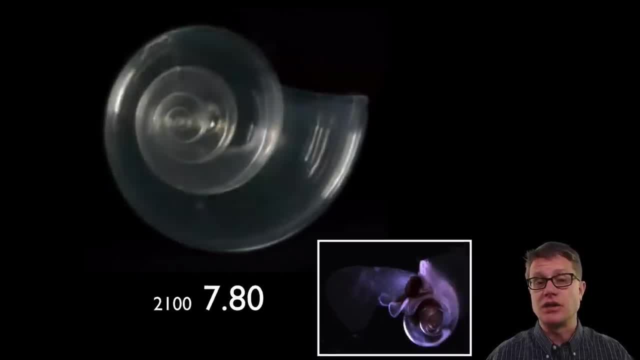 The free hydrogen is competing with that calcium carbonate to form more bicarbonate, And so now shells cannot make their shells. If we look at what could happen over time, this is a pteropod shell. at 7.8 pH It is literally going to dissolve. And so if we look at for 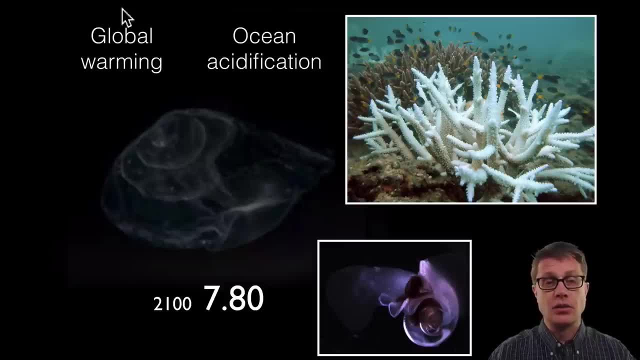 example, coral reefs. they are getting hit with a double whammy. We have got global warming. An increase in the temperature is going to cause them to bleach or kick out all of their algae. I will talk about that in a different video. But this ocean acidification is going.